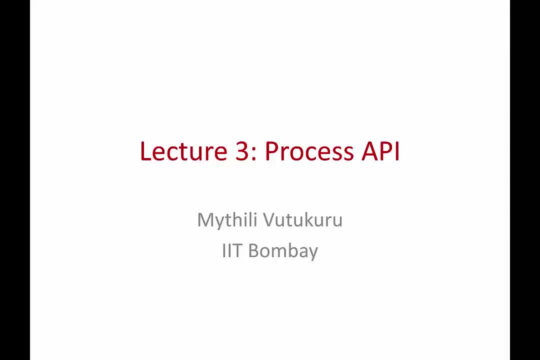 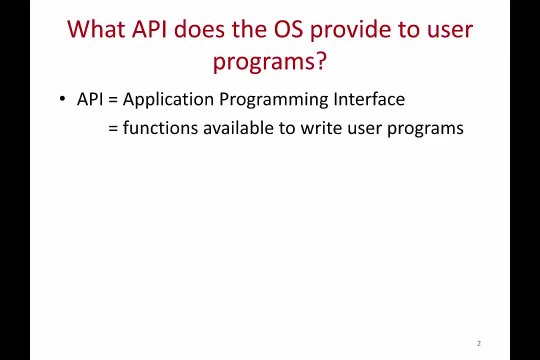 In this lecture, we are going to study the API that the operating system provides to user programs in order to create and manage processes. So what is an API? An API stands for Application Programming Interface, which is simply a fancy way of saying the functions that are available to users to write user programs. 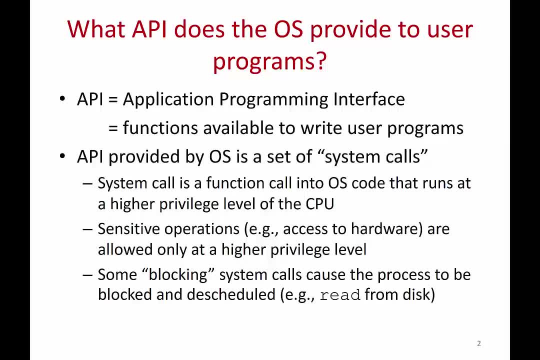 So the API provided by the operating system is basically a set of what are called system calls. So what is a system call? A system call is a function call into operating system code that runs at a higher privilege level. So a system call is like a function call. but 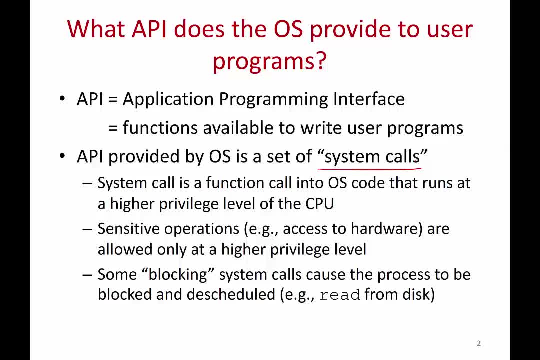 it runs with certain extra powers that regular function systems don't have. We'll understand this in more detail as we go along. And the system calls run at a higher privilege level and they have access to certain sensitive operations, For example, reading from the disk or accessing memory or allocating memory. 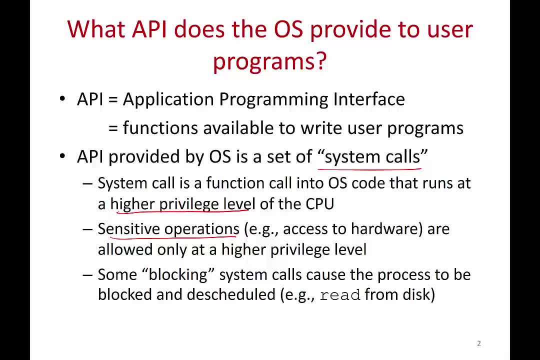 all of these are only allowed in a system call And that way it is different from a function call. And also some system calls are blocking That is when you make the system call, the process can no longer run and the operating system will take. 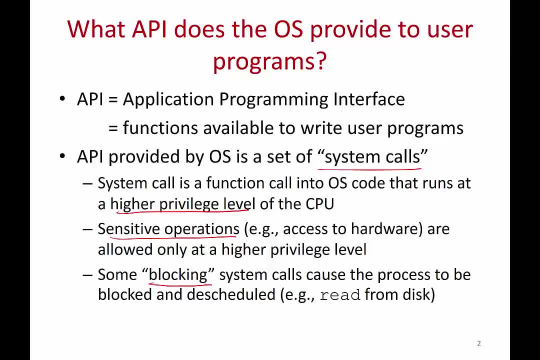 you out from the CPU. For example, if a process asks the operating system to read a file from the disk, say right, In that case the operating system, the system call, is set to block the process. right. So the API by the operating system is basically a set of system calls. 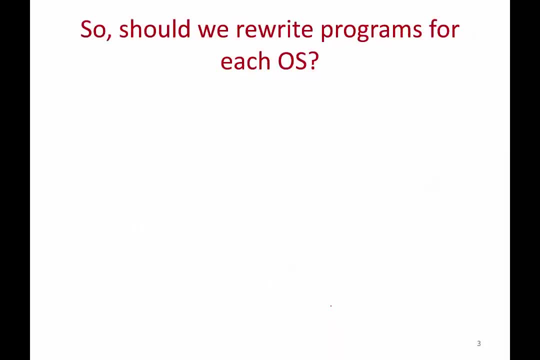 a set of functions that are available to user programs. So, given that these operating different operating systems can provide different system calls, does it mean that you have to rewrite your programs for every operating system? Because that would be a huge pain, right? If you have a C program, do you have to rewrite it when you 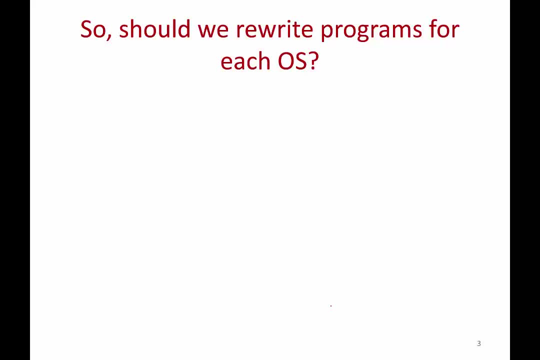 go from, say, Linux to Windows. Well, luckily that is not the case, for several reasons, right? The first thing is there is something called the POSIX API, right? So this is a set of common system calls that all the major operating systems have agreed on. So all the major operating systems. 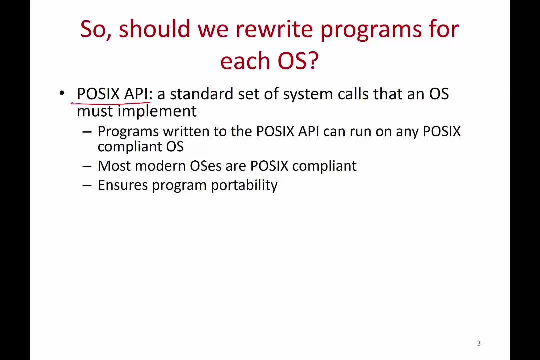 are compliant with this API. The second thing is that the POSIX API has the same set of system calls, the same API, which is known as the POSIX API, And because this API is the same, you can take your program and, without rewriting, run it on any operating system that supports this. 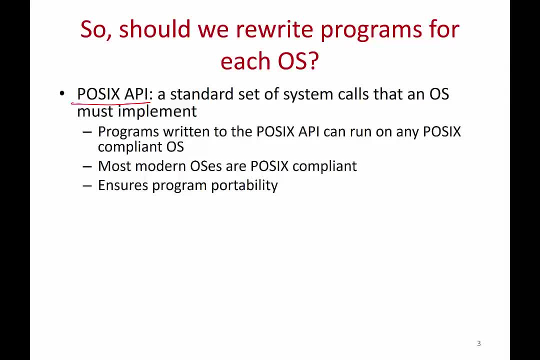 API right. Almost most modern operating systems are compliant with this API And this is really a key factor in ensuring that programs are portable across different systems And you don't have to re-write the system calls when you move to a different machine And there's also another. 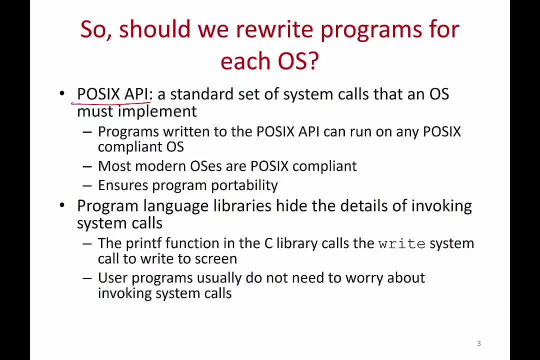 reason that makes life easy, which is it is very rare that a user program will invoke the system call directly right. Most of the time, program libraries, for example the C library, provide certain high-level functions and these functions in turn invoke the system call right. 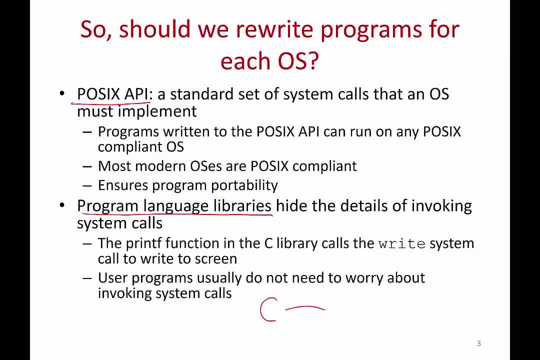 So the user is almost never directly invoking the system call. For example, your C program might invoke some function from the C library which in turn invokes the system call, so that you don't have to worry about knowing what the system calls are and calling them in your code, For example if the program wants to write something. 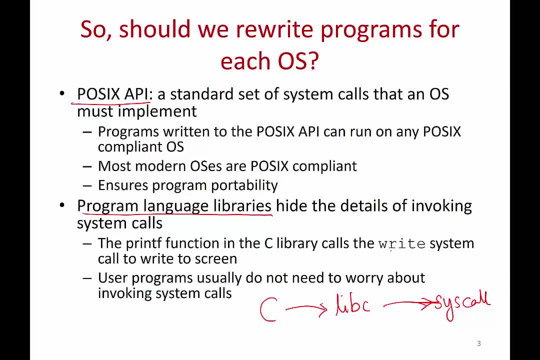 to the screen, right? The correct way to do it is to use the right system call to write to the screen, but this is a little cumbersome, So instead you will use the printf function that is provided by the C library, and this function, in turn, will make the system call for you. okay, So the high-level 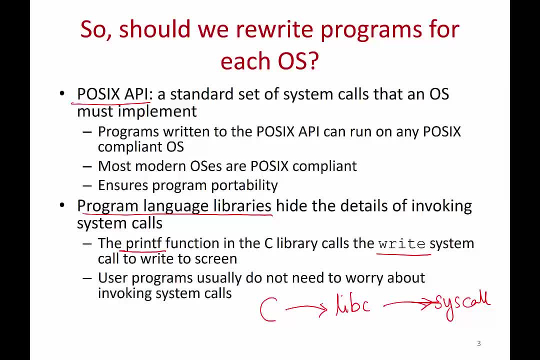 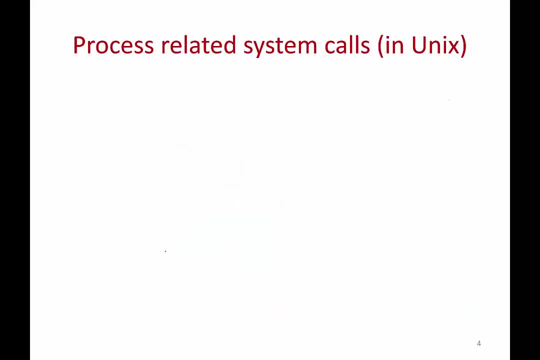 system call is: the operating system provides a set of system calls for users to write programs, but you don't have to worry about invoking them because the library program language libraries take care of that for you. So we'll begin with a discussion on what are the system calls related to creating and managing. 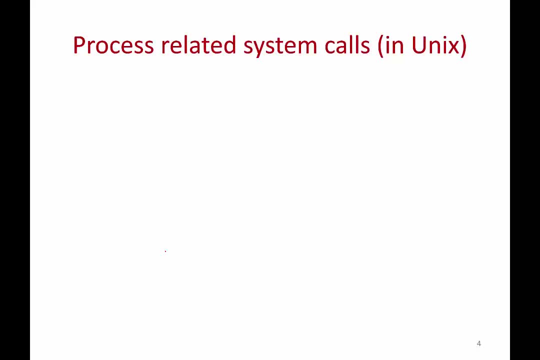 processes in Unix-like systems, for example in operating systems like Linux. right In the rest of the course we're going to study a few other system calls. So the most important system call to create processes is the fork system call. So what? 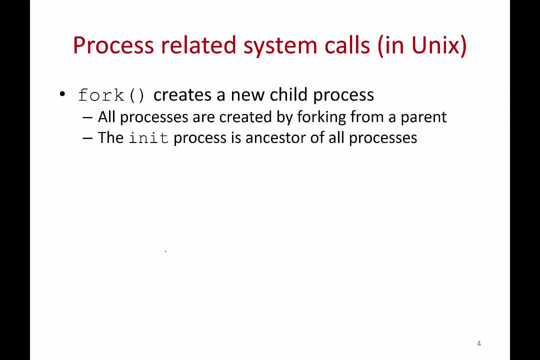 does fork. do Fork creates a child process from a parent process. Note that there's no way to create a process just on its own. Every process is created from another process. So the operating system, when it starts it, creates what is called the init process. 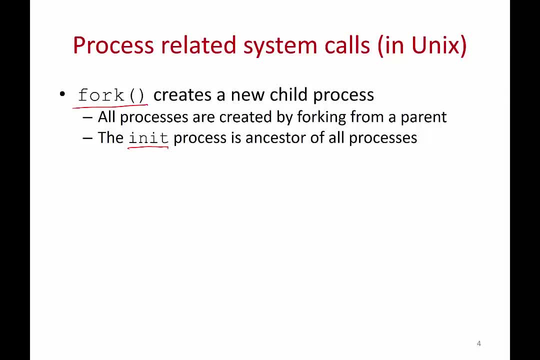 and the init process forks off a few other processes, which fork off a few other processes, and so on. Okay then, if you want your process to execute a certain executable, you use the exec system call- We'll come to this in more detail- And if a process wants to terminate, it uses the. 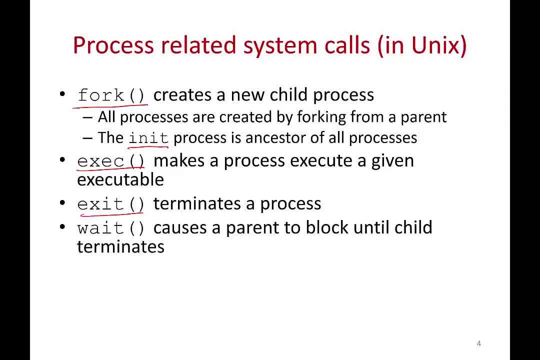 exit system call And if a process wants to wait for certain events- for example, if a parent wants to wait until the child terminates- it uses the wait system call. We're going to study all of this in some detail And many variants of all of these system calls exist. There are different ways of invoking exec. 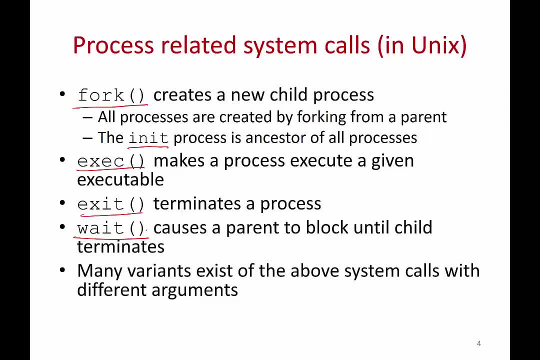 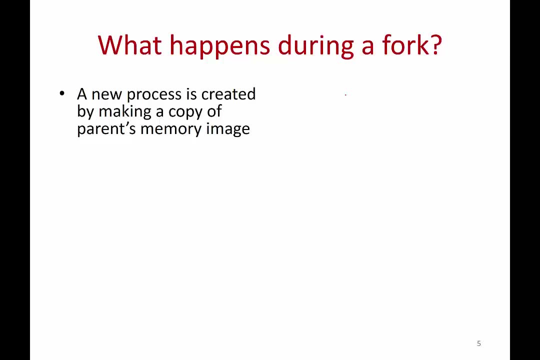 and wait and all of that. So fork exec, wait. these are the most important system calls in Unix-like systems to manage processes. So let's study in some detail what happens during a fork. So here you have a parent process. Let's call it P. It has a certain memory image. It has some code. 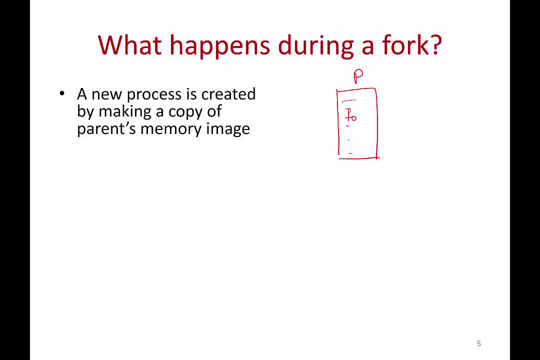 Right, And this process? in the code it makes a call to fork: Okay. So then what happens? The operating system makes a copy of this parent, creates a new process by making a copy of the parent. Let's call this the child process, C. Okay, and C's code is an exact copy of the. 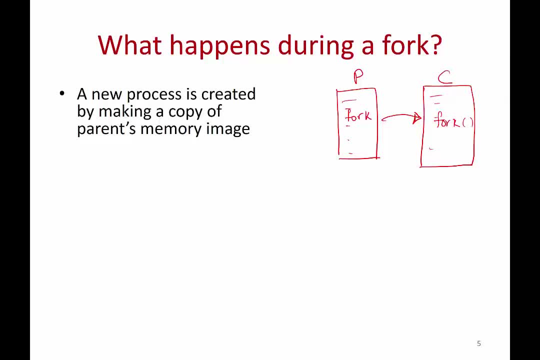 parent's code: right, There's the line fork, the fork call. everything is there in C also in the child process process also, and this new process, now remember, the os has a list of, you know, a link list of processes in the system and this process c is also added to this list, right, so that the os 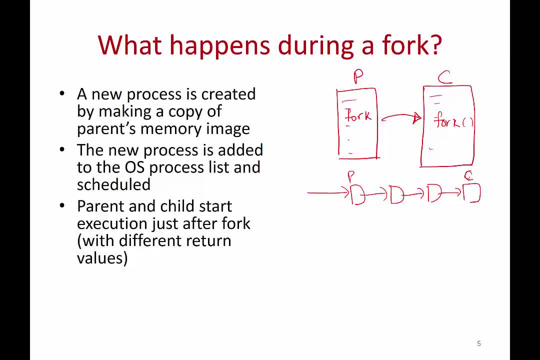 can keep track of this process and both parent and child are now scheduled and they execute independently. sometimes p gets the cpu, sometimes c gets the cpu and so on. right, and both these processes they resume execution from the same point at the fork statement. just that, the return. 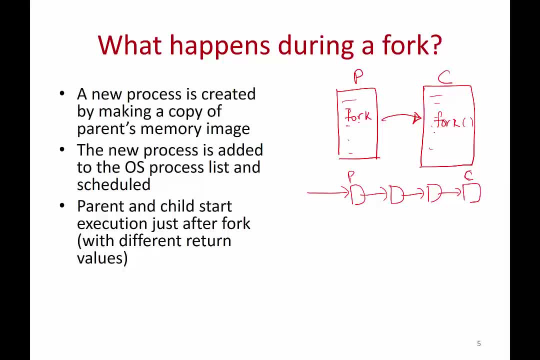 value from fork is different. we want to see that in just a little bit. but when you fork a copy of your entire code data, everything is made in the child and both the parent and the child are added to the list of processes and they keep executing. note that the child's memory is a copy of the 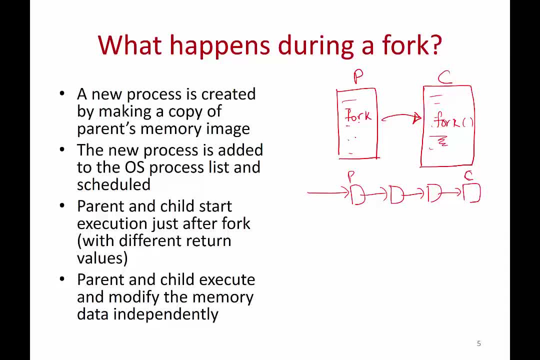 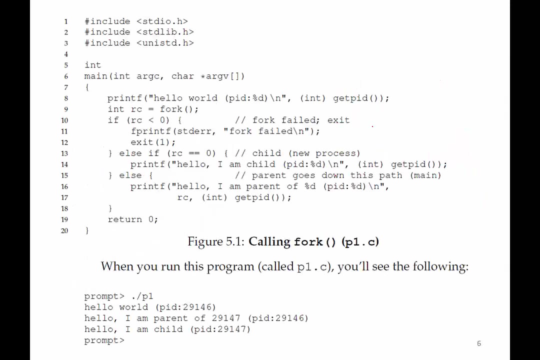 parent's memory initially, but the child can go on make, keep changing its memory. the parent can keep changing its memory independently right once after the fork. the parent and child are two independent processes that are running on their memory images which just happen to be a copy of each other during creation. so here is a small example code that uses the fork. 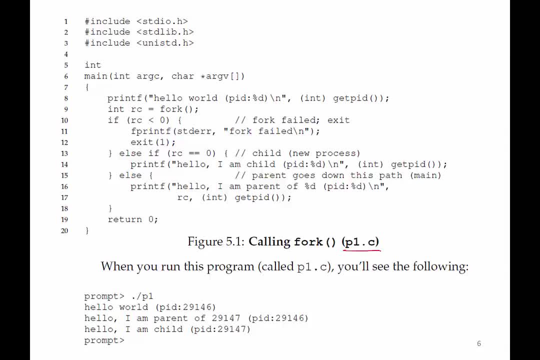 system call: right, so here is a process p1.c and this process calls for: okay, so when it calls fork, here is your p1.c that is running a process. and when it calls fork, an exact copy of that is made into another child process, right? and if you see the 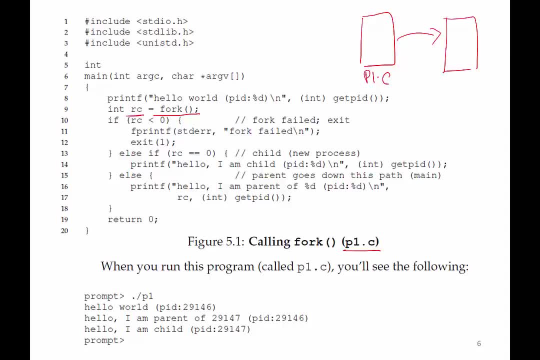 return value from fork right, this variable rc. this return value is set to different values in the parent and the child. both of them have the same variable, but it is set to different values in the child. this return value is zero, right? so whatever code goes into this, 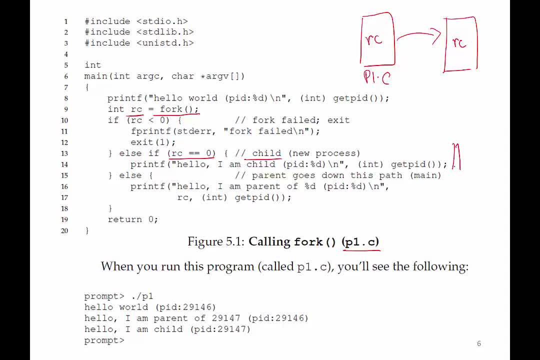 rc equal to zero. this code is the child code, okay, and this value of rc is non-zero in the parent. so whatever is there in this part, this is the parent process, which is the return value from fork is actually the pid of the child in the parent. therefore, the 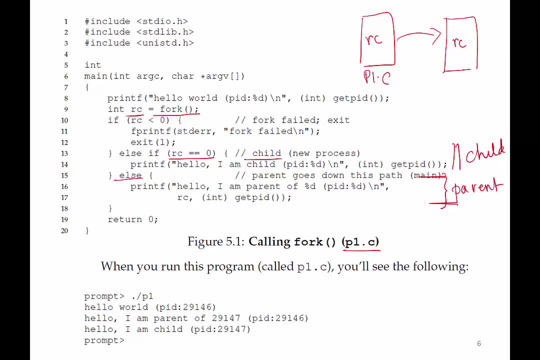 parent process, which is looking at the return of the child. this is not necessary because we canımız the per by ina example output, which is the screen. but these are. this is output from two different processes, the parent and the child, with both happen to be running the same code, with different parts of the code. 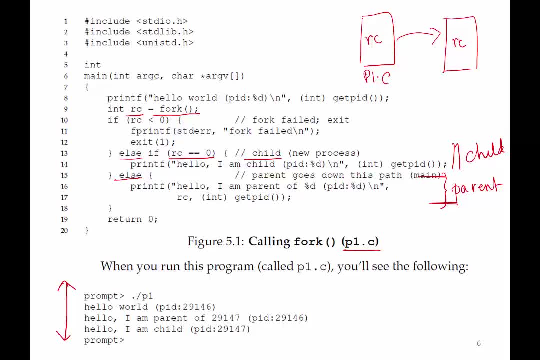 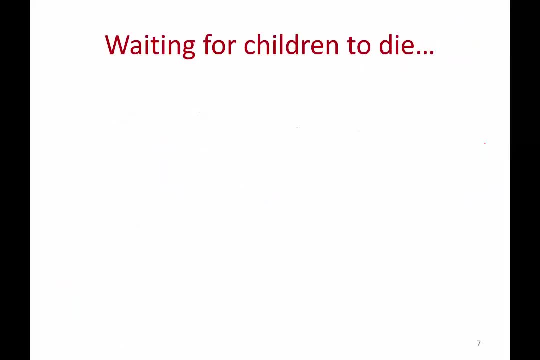 because the return value, the rc variable, is different. right? so next we come to the relationship between parent and child processes and what happens when the child process terminates and the parent process terminates, and so on. so the title is a little scary, but let's go into the details. so when a process terminates, what happens? so how does? 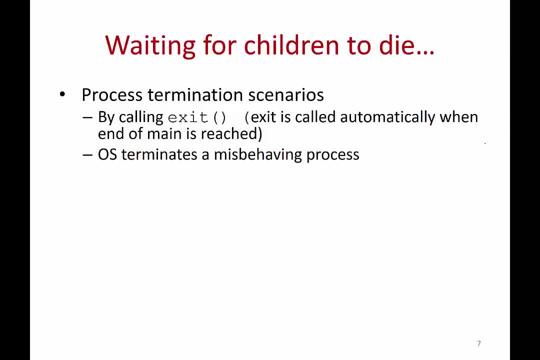 the process terminates, it can just call exit and terminate itself normally. for example, when you reach the end of the main function, when you're finished executing all your instructions, the process terminates normally. or if a process does something stupid, does some something illegal, the os can terminate the process. right, there are two ways of terminating. 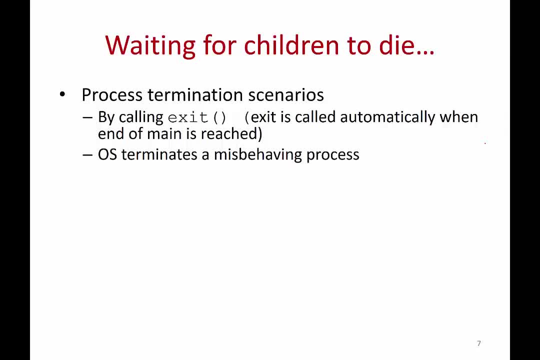 a process, a normal scenario and an abnormal scenario. so, whatever the way the process terminates, what happens, these terminating processes are not immediately removed from the list of processes. instead, they exist as zombies. right, and when is a zombie process finally cleared out? when the parent calls wait, right. so 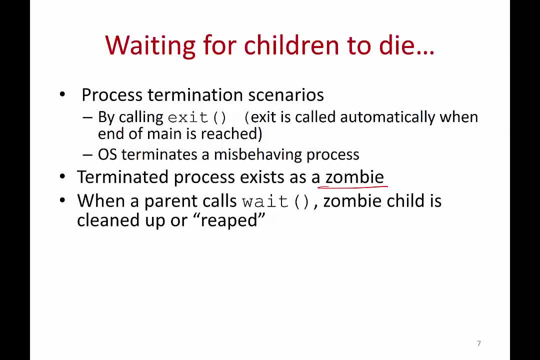 somebody has to. a parent has to clean up or reap a dead child. only then is a process truly cleared out of the system. okay, and this wait call blocks in the parent until the child terminates, right. so when a parent calls, wait until the child finishes execution, the parent will block. it will not. 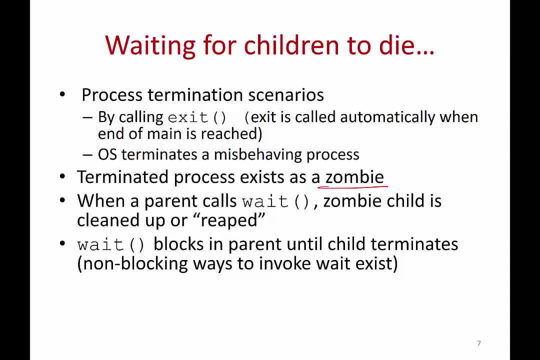 proceed further. of course there are ways of you know, calling wait without blocking. we'll come to the next slide, and so now the question comes up right. so here is a parent process that has spawned a child and until the child terminates, the parent has to wait. right, when it calls wait, the parent 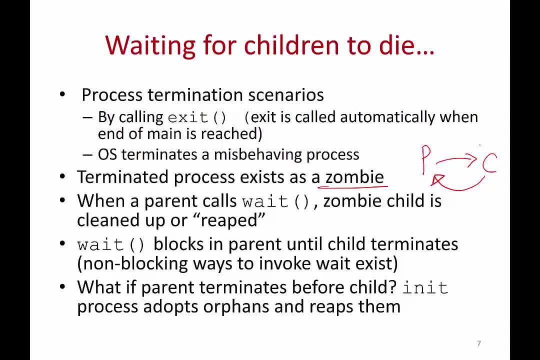 blocks until the child terminates, okay, and when the child terminates then the wait system call returns in the parent. but suppose by the time the child has terminated the parent no longer exists. what if the parent has exited, has terminated before the child? in which case what happens? who will clean? 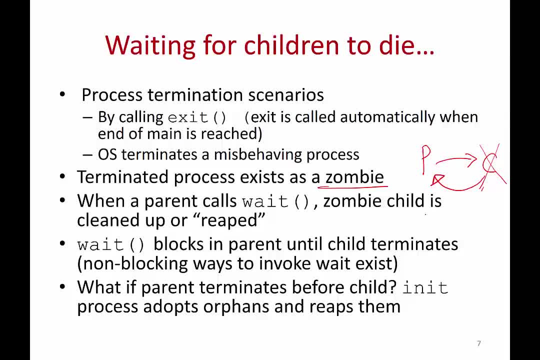 up the child. so in such cases, the init process right. the init process is the one that reaps all the orphans whose parents have died. so here is a process: P- it has spawned a child C and P has exited, in which case when C terminates, it is reaped. it is cleaned up by the init process. right, because 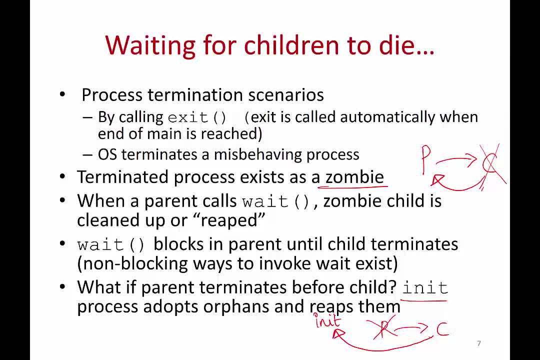 the init process is the ancestor of all processes and therefore all orphan processes whose parents are not around to clean after them. they will be reaped and cleaned up by the init process. so you may be having this question: why is this the case? right, when a process terminates, why can't its? 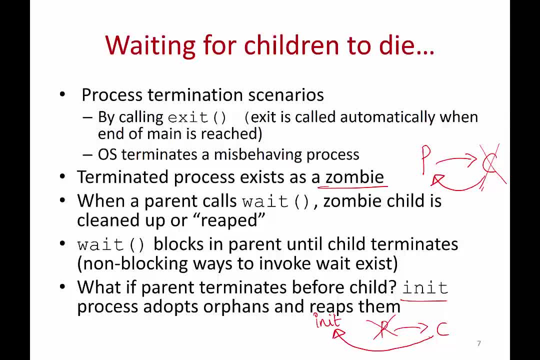 state be simply cleared out. why should the parent call wait and then clean up state right? there's certain subtle reasons for this that may be out of scope for this lecture, but just remember that any time a process terminates, somebody has to call wait and reap the process and clean up the process. otherwise it is going to exist as a zombie and 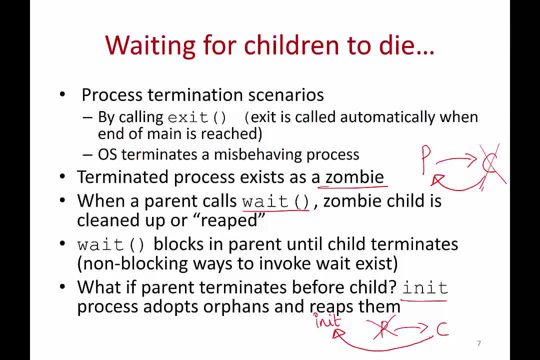 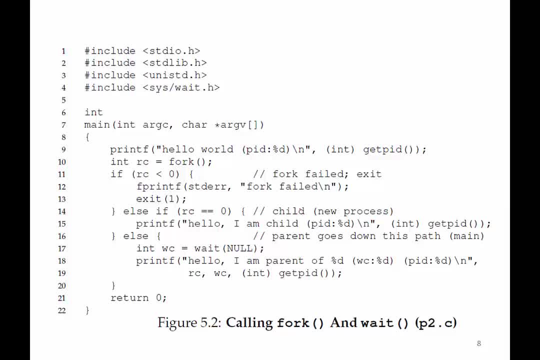 keep consuming memory, keep consuming resources in the system. so here is a simple example of a program that uses the wait system call. so this is the parent that has called fork right and here. so this return value of fork is zero here. so this is the child process, this code, the child. 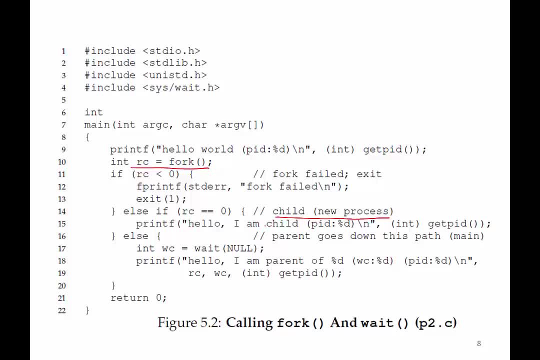 prints this. and once the child Prints this, hello, the child is done. and what does the parent do? the parent calls wait. so the parent process basically stops execution. the parent blocks here, okay, until the Child terminates. and when the child finishes, that is when the parent moves on from. 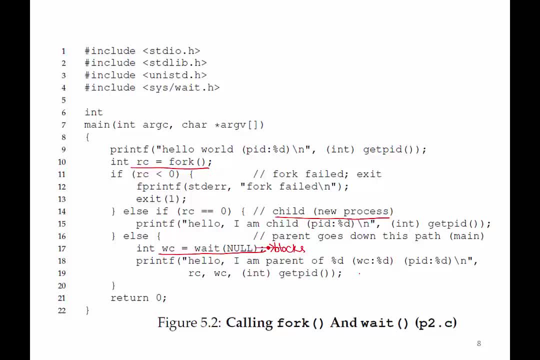 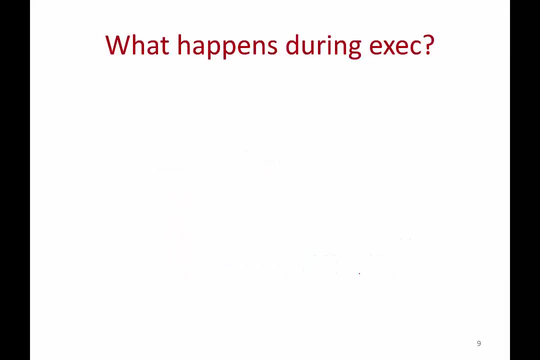 weight and prints this statement right is an example where the parent is waiting for the child process to clean up after it finishes. so the next system call we're going to study is exec right. what happens during the exec system call. so we've seen that after fork, here is the parent and here is the child. they're both running. 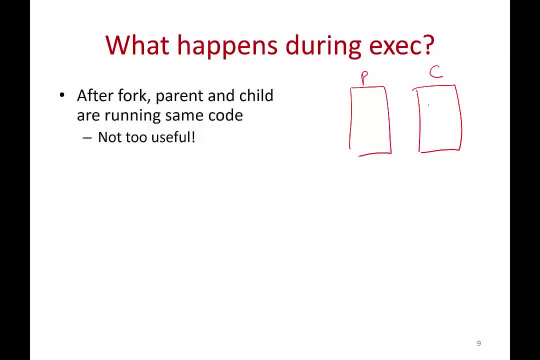 the copy of the same code right, it is the same program that the child is running. but this is not useful. what if the parent wants the child to do something else apart from its own code? right? in such cases we use the exec system call. so when the child process calls exec right, what happens? its? 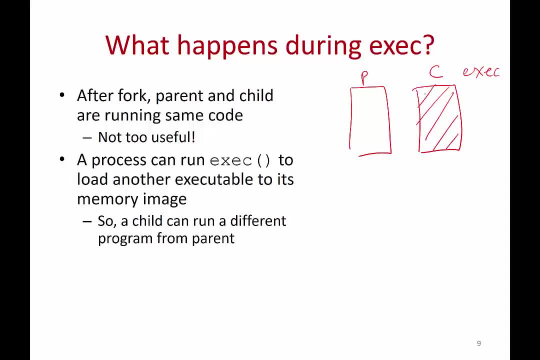 memory image is replaced by another executable. it is no longer running the executable, the code of its parent, but you can run a completely different executable in the child process. right, you will get new code, new data and everything new, right? so you reboot as a new process. so that is the exec system call. 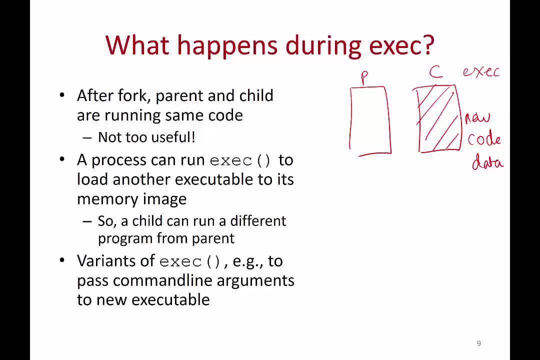 and there are several variants of exec where, when you're running this new program, you can give it some arguments, you can do all sorts of things, you can set up this new process any way you want. right? so this is the exec system call, and here is a small example. right so this is again similar. 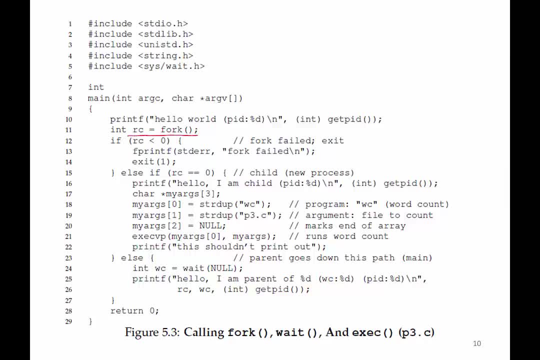 familiar code. here is the fork statement. a parent has spawned a child process and here is the code for the child process. right, so the child process no longer just wants to run the code of the parent. instead, the child process calls exec. this is a variant of exec. accept vp here, but this variant 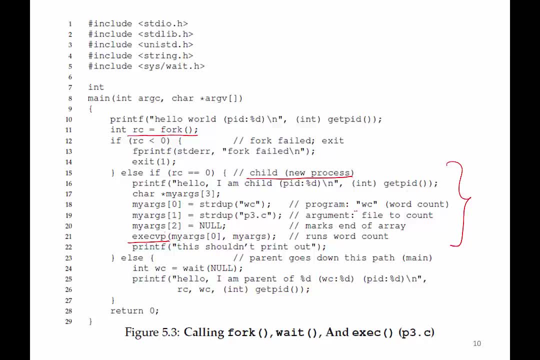 basically runs some other program. right, it runs the word count program. you can run whatever program you want. you can pass arguments to the program, right, and so the child process is now Rush分 Kin, no longer running this code, but it is running. it's doing something completely different. 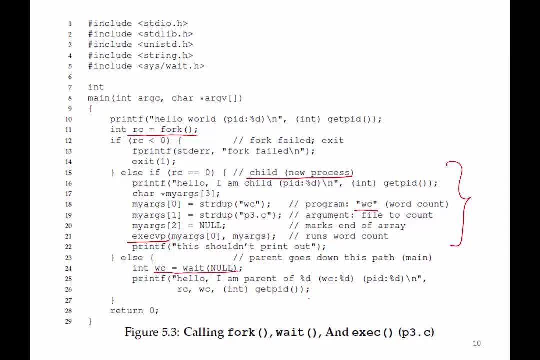 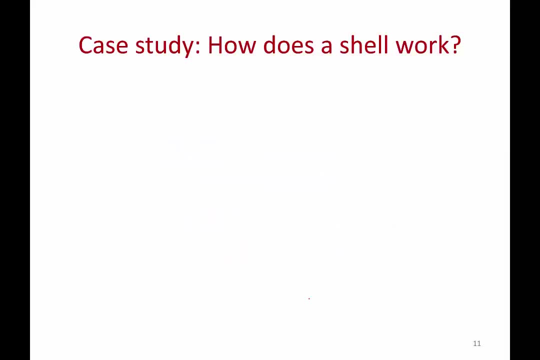 whereas the parent process is once again waiting for the child and exiting. so the fork exec wait system calls are very important, and we're going to study how a shell works in order to fully wrap our heads around these system calls. so what is a shell? in any basic operating system, the init process is created right after. 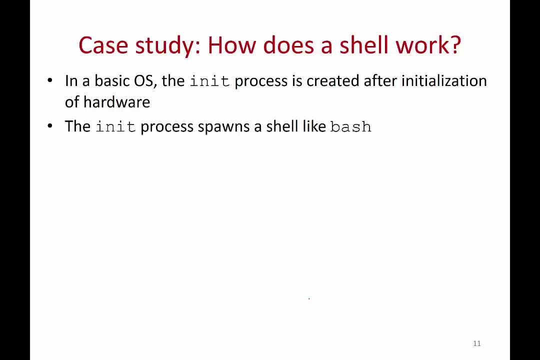 initialization and it spawns a whole bunch of processes, and one of which is a shell, like the bash shell, right? so when you boot up a system, you get a command prompt. that is what comes from the shell. so what is a shell? it is something that takes user inputs and executes programs on behalf. 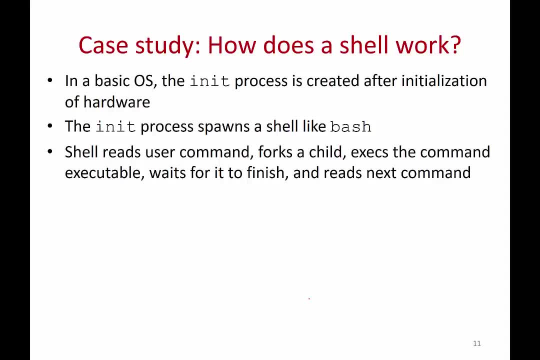 of the user. so what does a simple shell do? it gives out a prompt and the user can type a command. it reads the user command and then how does it execute the command? it forks a separate child process, execs, call execs in that child process to run the command, waits for the child. 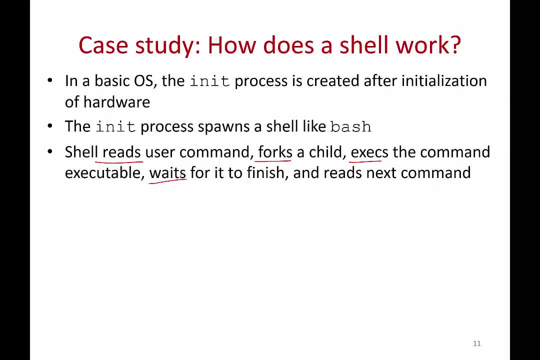 process to finish and then goes back to the user to read the next command. right, so all common commands are just like ls, are all available as executables in an operating system, and these are all exact by the shell, for example. let's see what happens here. right here is a command. 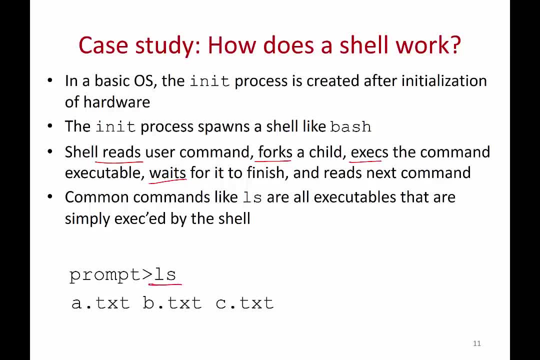 prompt and you've typed ls at the command prompt. so what is happening? you have your shell process that has, you know, asked the user for an input. the user has typed ls. so then, what does shell do? it forks a child process and then it calls exec on the child process, giving this ls as the program. 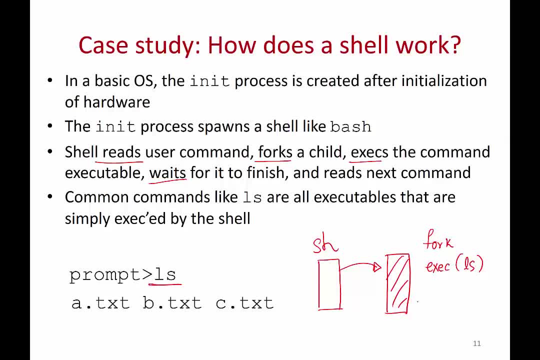 to run and once the child process finishes running ls, it prints out the output from ls and the child process terminates. then the shell calls wait, waits until the child process finishes and then finally it comes back to the user and says: give me the next command, right? so if you build a simple shell, you'll really understand how these 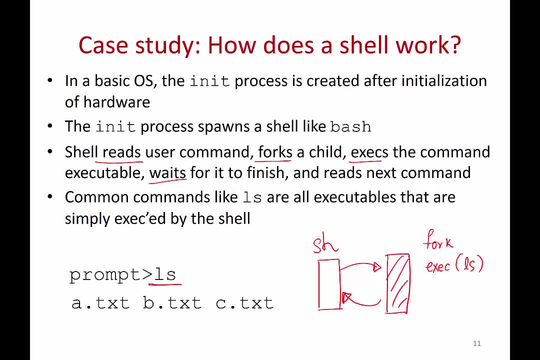 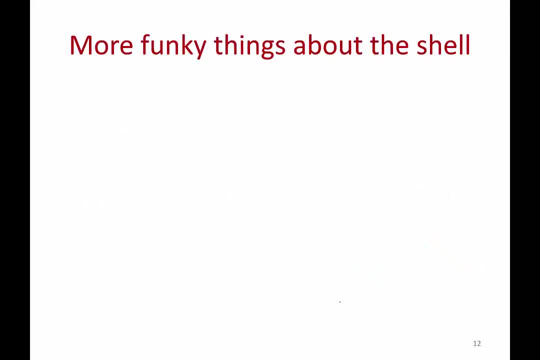 wait for exec. all of these system calls work, so the shell also does a lot of other funky things right. it doesn't. so what we've seen is the simplest use case for the shell. so the shell can also manipulate this child process in many different ways. for example, if you want to redirect the output from a command to a file. 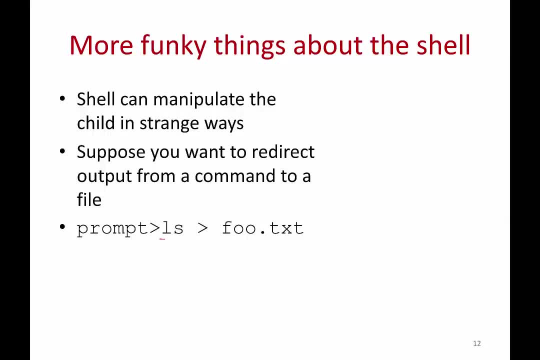 right, you want to do something like this. you want to run ls, but you don't want the output to be displayed to the screen. you want to store it in a file. so this is a common thing that many of you would have done. so how does this work? so the shell spawns a child process, as before. here is the shell. 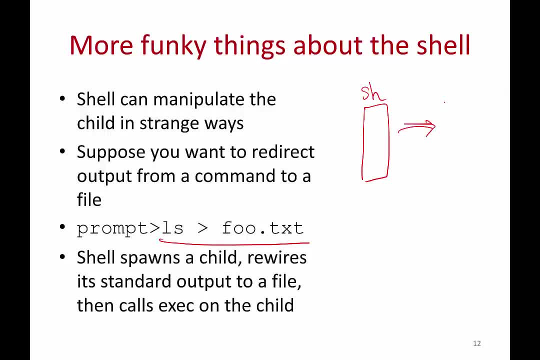 process, it spawns a child process. and then this child process has certain. you know its standard input, standard output. everything was pointing to the screen, right? so then it says: don't write to the screen. instead, it changes the output file descriptor and makes it point to this food or text. 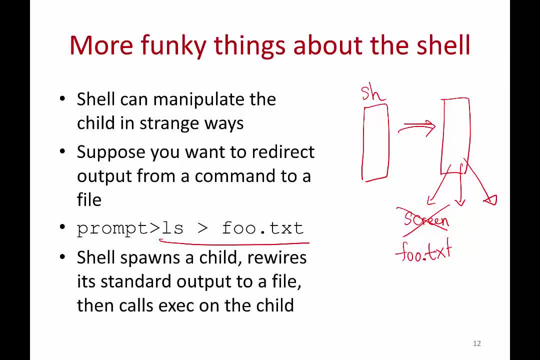 it manipulates the child so that its output is not going to the screen but going to food or text. and then it runs exec. it copies the ls executable on the memory image of the child, right. so by doing this, when the child process runs, it no longer writes output to the screen, but it. 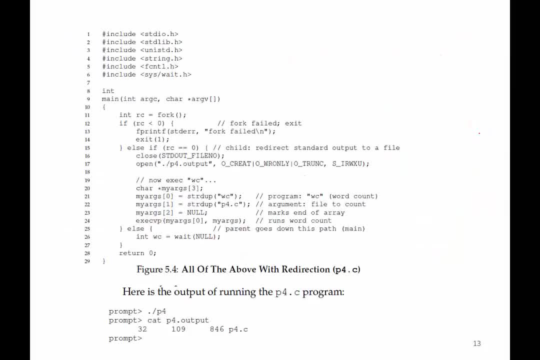 will write it to food or text. so here is some code that actually does that. so this is your parent shell process that has forked. and then in the child right here is your child process. now the child process. you close the standard output. you no longer write to the screen and instead you open another output file. here you close standard. 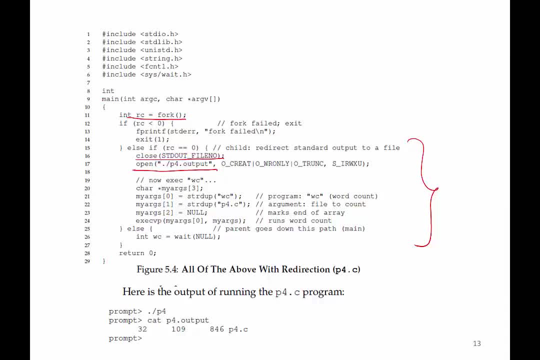 output and you opened something called p4.output. you've opened that file so that instead of writing whatever was going to the screen, to the standard output, will now go to this p4.output. okay, and now the child execs this word count command. so what happens when you run this code? so when you run,